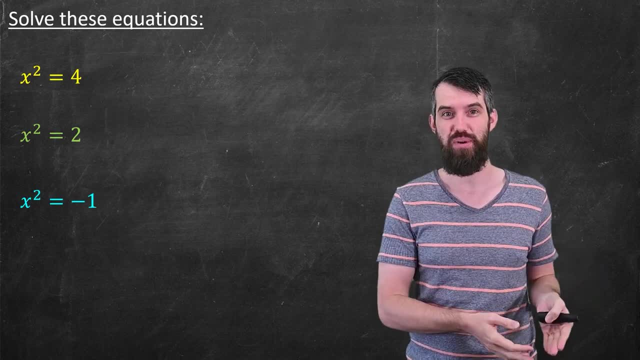 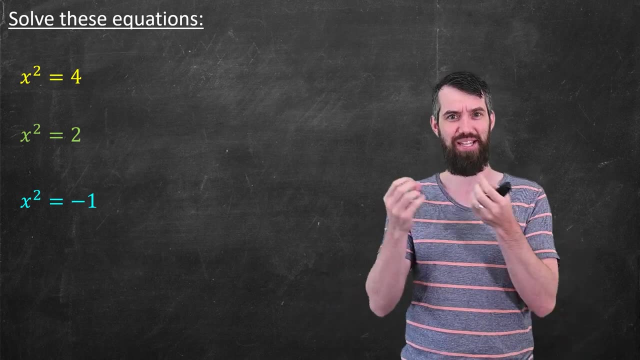 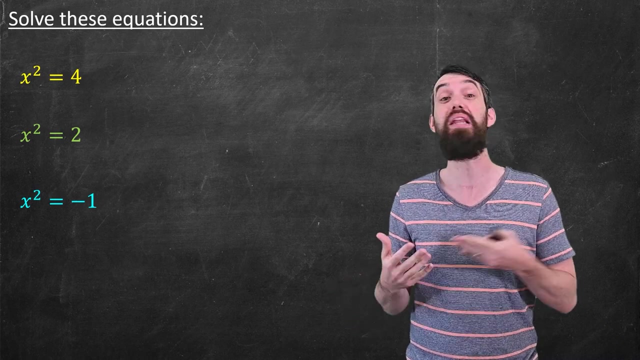 Welcome to my new series on complex and imaginary numbers. Over the course of the next couple of videos I want to convince you that, despite the kind of mystical names- complex and imaginary numbers- that these objects in mathematics are actually very natural and powerful tools to solve many different types of problems in mathematics, science and engineering. 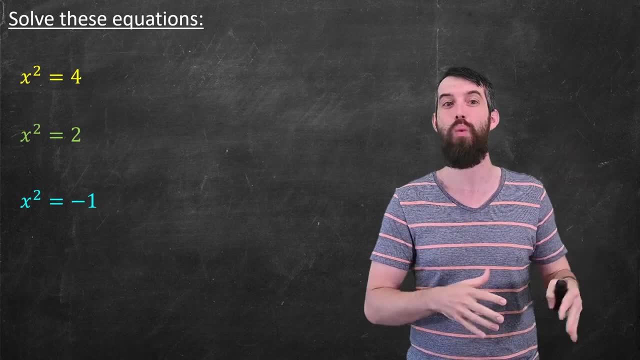 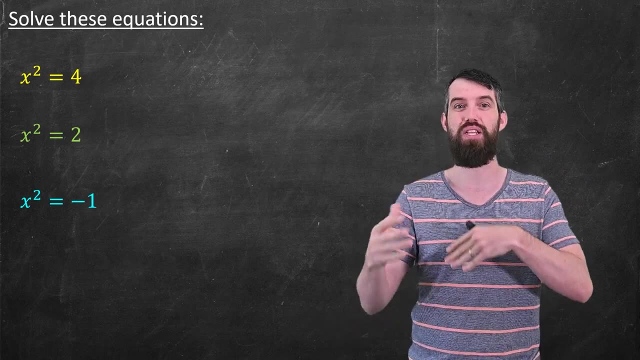 In this first video we're really going to focus on an algebraic picture: why we think that complex numbers are helpful to us algebraically and some of the advantages that complex numbers give. In the next video we're going to talk about the geometric picture of complex numbers And then 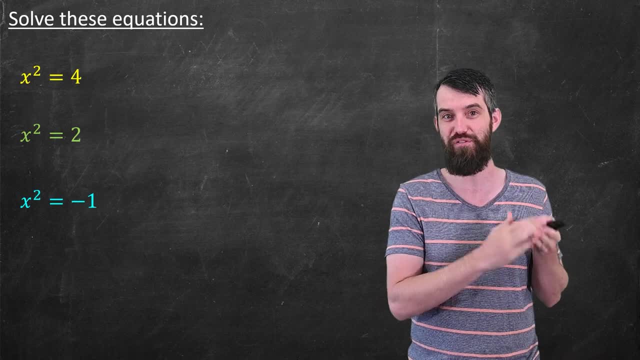 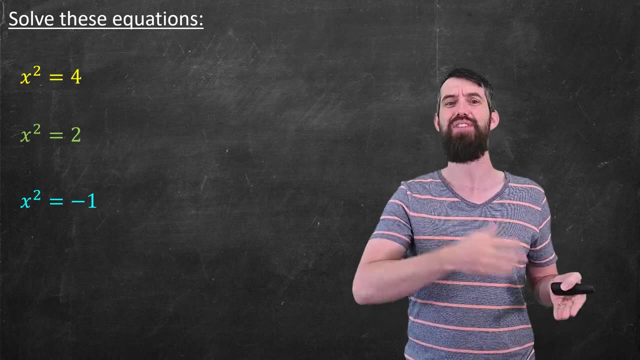 finally, in the third video we're going to talk about a very powerful feature of complex numbers, which is writing them in polar form. It's going to make our lives a lot easier and allow us to have nice answers to things like: what's the cube root of minus one? 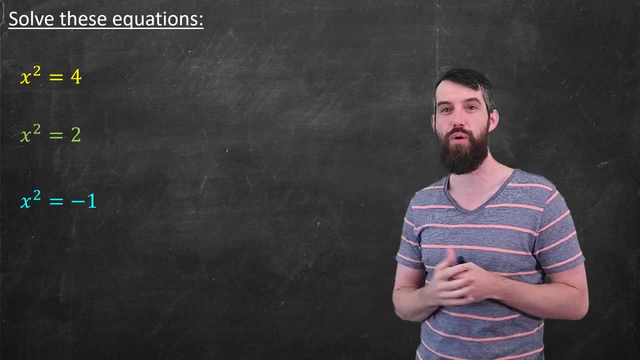 All right, so let's begin with these three different equations: x squared is four, x squared is two, x squared is minus one. And the question is: can we solve them? Well, the first one is: how do we solve them? 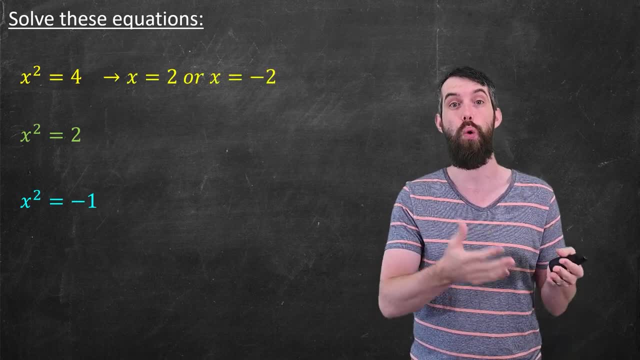 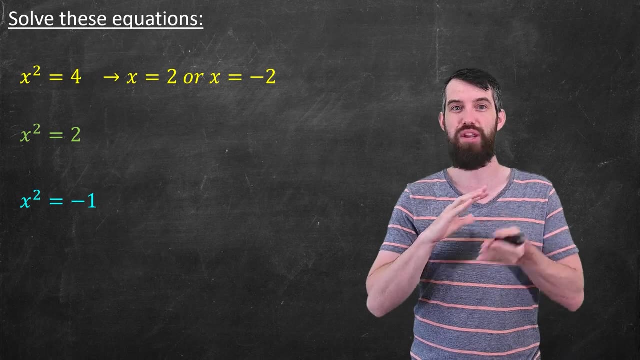 The first of these is straightforward. The solution is: x is two or minus two. You plug either of those numbers in, you square it and you get four, Because two and minus two are integers. I don't think anyone probably has a problem with that, But maybe you do with the second one. 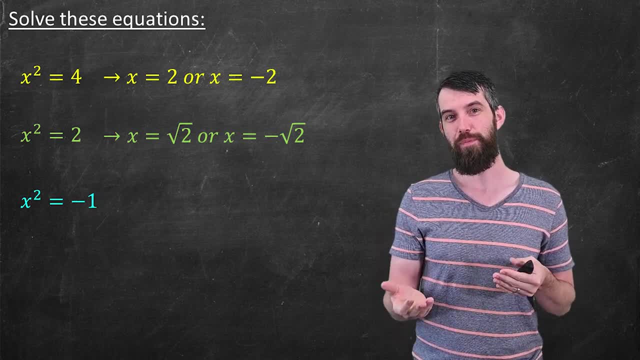 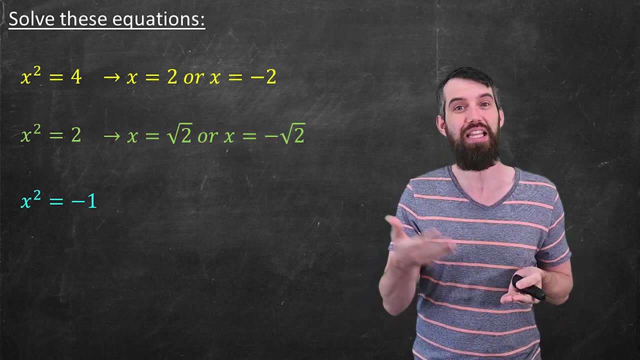 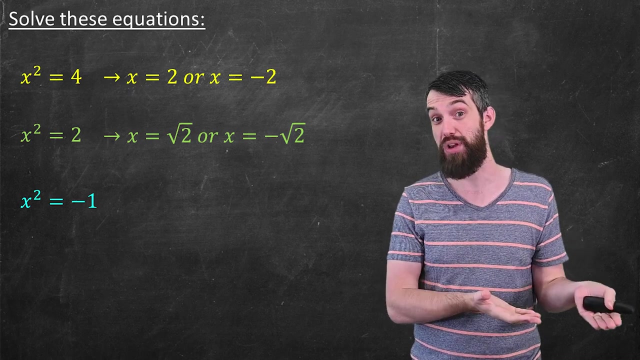 The second equation: x squared equal to two. well, when you solve that, I can write down x's square root of two and x's minus square root of two. But what really is the square root of two? Indeed, square root of two is a very bizarre thing. It's not a rational number. You can prove that It's. 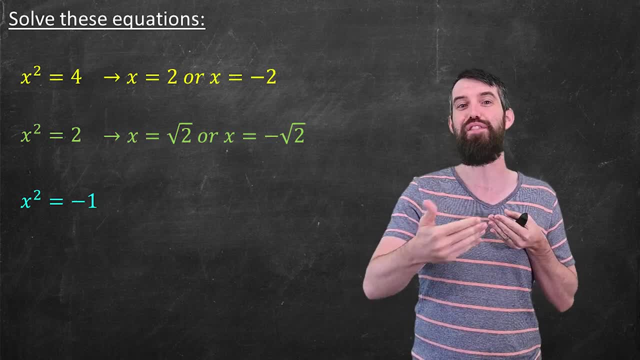 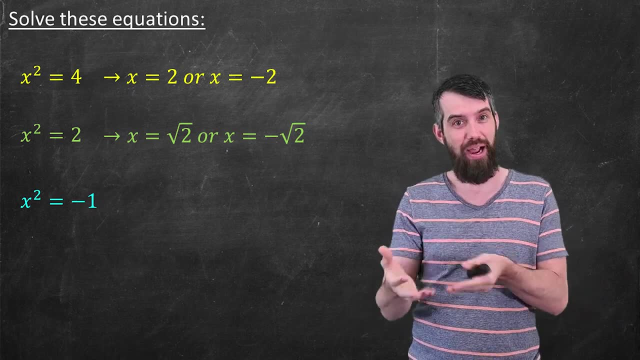 not a fraction like three over seven is. It's something with an infinite, non-repeating decimal expansion, But does that even really exist? So the idea is that the symbol root two and minus root two, these things are definition. They are defining the concept of the number. that is the 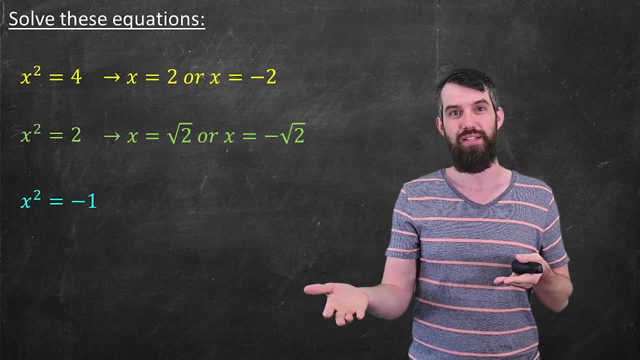 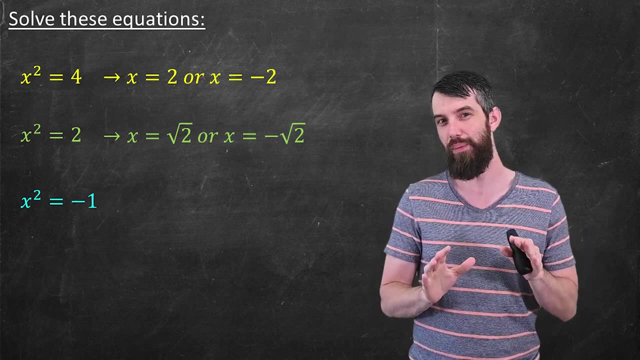 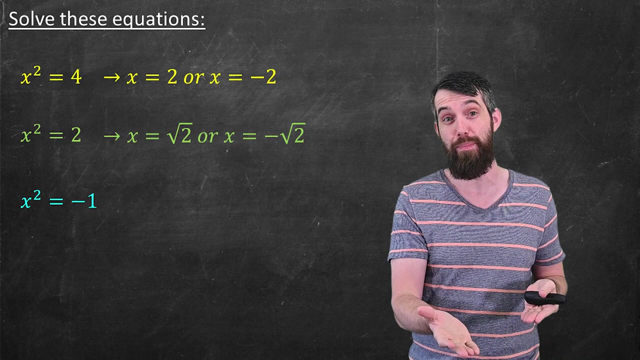 solution to x squared equal to two. So there's already a little bit of a mystical- we're sort of defining things kind of thing going on. So if you're happy with that, you're happy with the idea that we can define solutions to equations, then perhaps you'll be also happy with the next one. 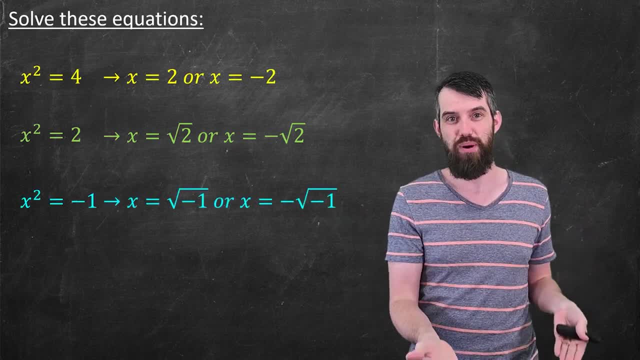 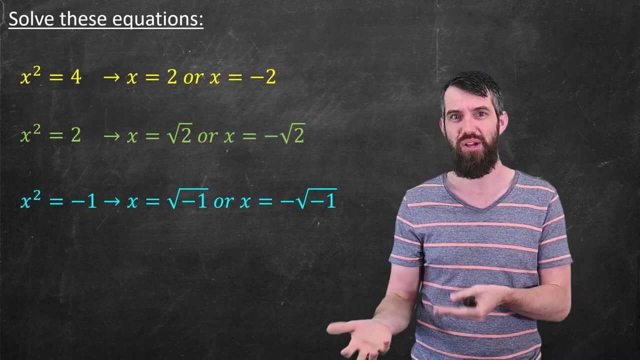 the solution to x squared equal to minus one. If I take square roots of both sides, that would give me x equal to square root of minus one and the negative square root of minus one. Now, when you square a real number like seven squared is 49 and minus seven squared is also 49, whether it's. 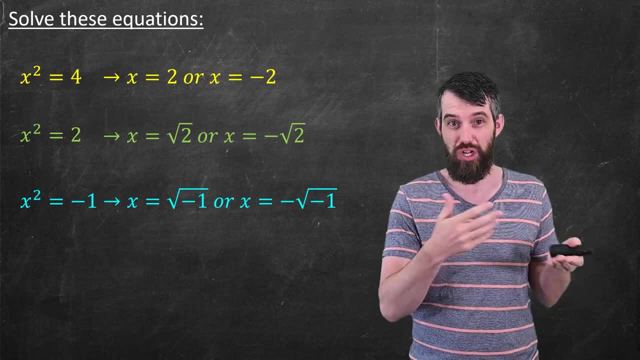 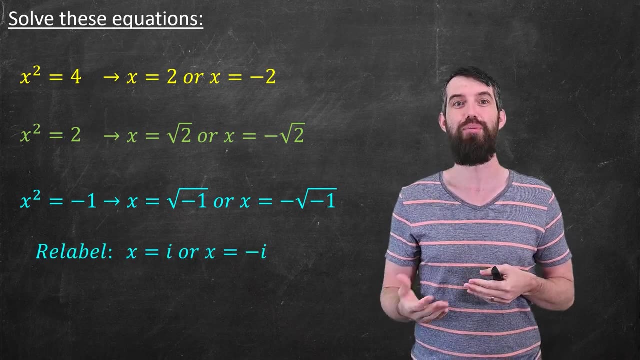 x squared to a positive. So the square root of a negative number should cause a lot of anxiety to you, But I'm just going to define it to be something. In fact, I'm even going to relabel it because it's going to be important enough. I'm going to relabel the square root of minus one. 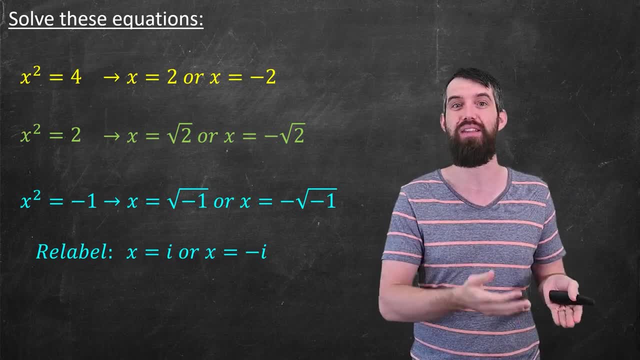 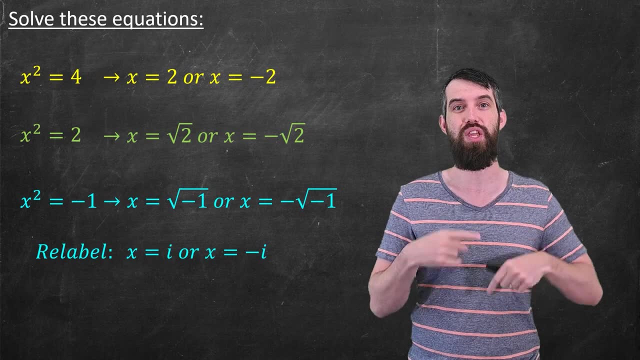 and give a shorthand to that symbol and call it instead the symbol i and minus i, And what I'm really doing is just defining this new symbol i or negative i to be the objects that solve the equation x squared equal to minus one. I'm sort of continuing my analysis of the equation. I'm 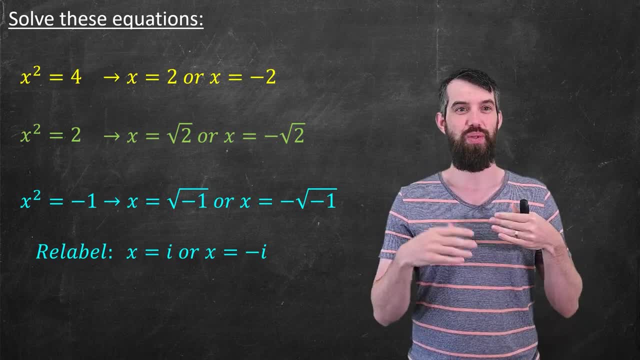 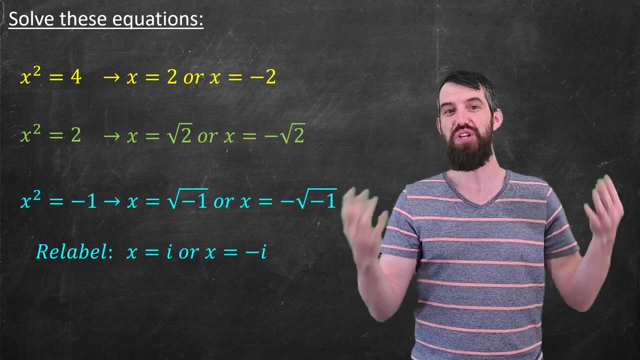 going to give it an analogy with the way we came up with root two. So you might be left with the impression that if I'm going to be comfortable doing that, that the cat's kind of out of the bag and we're going to have a huge number of new symbols we'll have to define. For example, if I 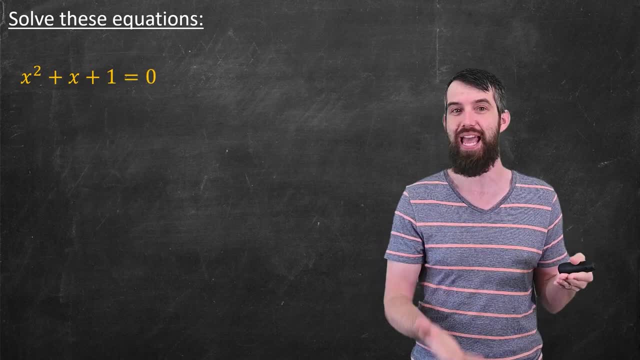 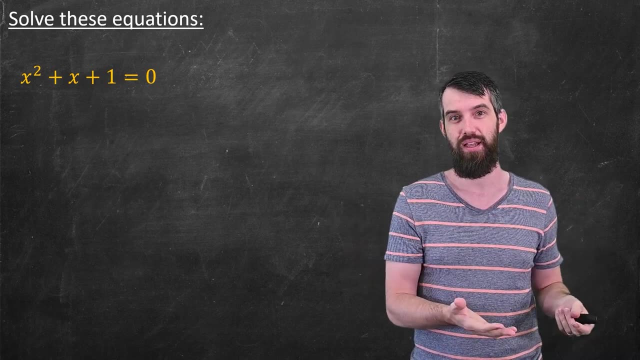 consider some other quadratic equation. how about x squared plus x plus one equal to zero? Okay, well, maybe you'll have to find some new symbols yet again for the solutions to this. Except, this has a quadratic formula. We could plug that in and get x is well, normally it's minus b plus. 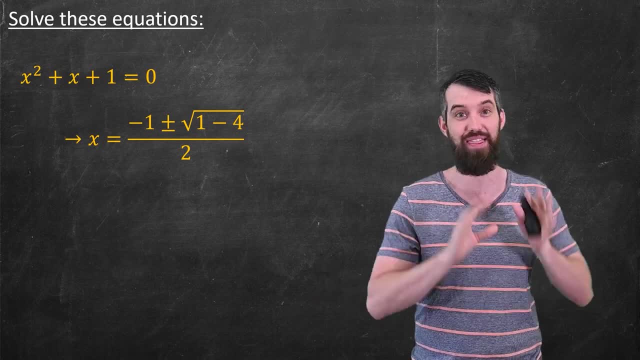 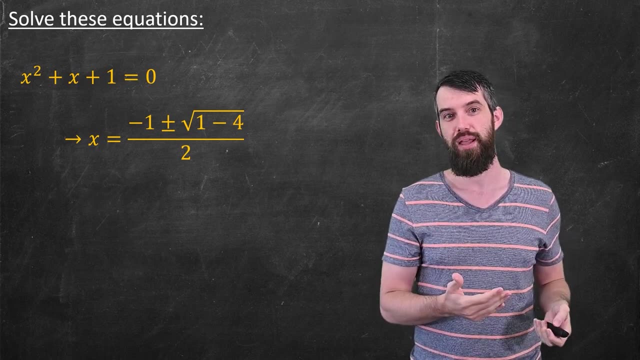 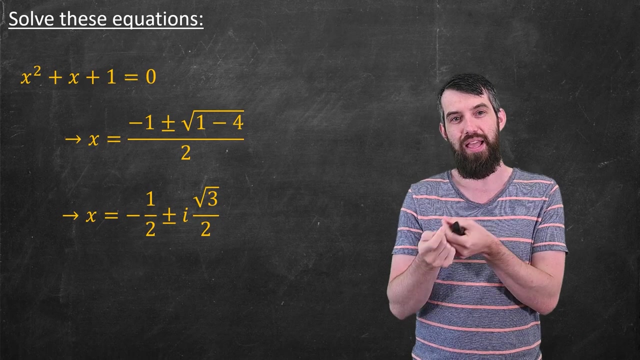 or minus the square root of b, squared minus 4ac, all divided by 2a, That formula. So in this case minus one, plus or minus square root of one minus four, and then divided by two, And then, if I just simplify that a little bit, okay, one minus four, here is negative three And then square root of. 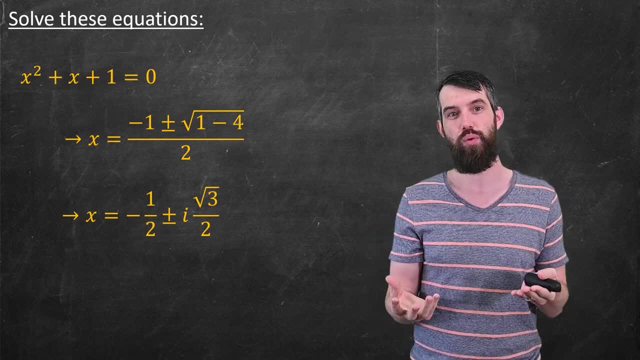 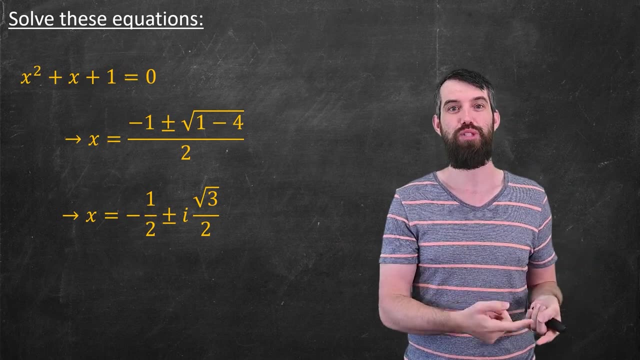 negative three can be thought of as square root of minus one times square root of three And square root of minus one we have defined to be i. So what do I get? Negative one half plus or minus square root of three divided by two. The point here is that I haven't had to come up with 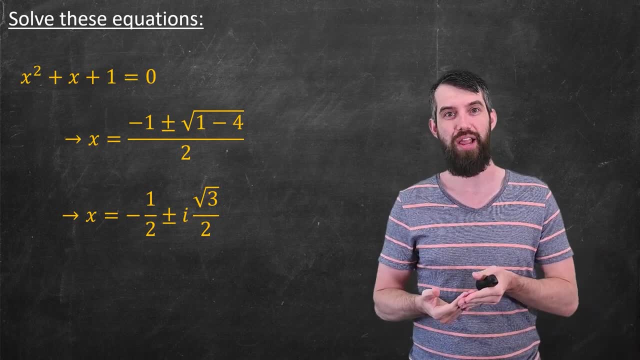 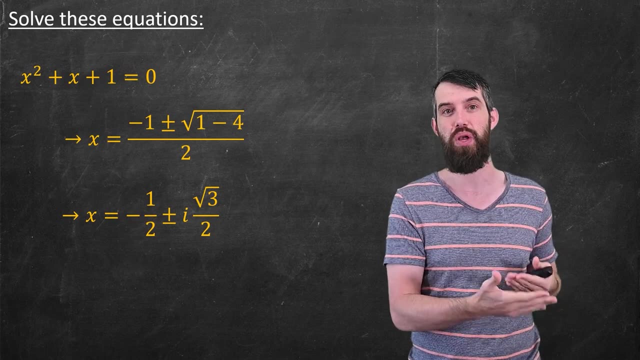 yet another new symbol That the i I already defined was enough. By the quadratic formula I got this thing with the square root of minus one, but I'd already defined that thing to be this symbol that we call i. Now I'll note that in this case there's a portion at the beginning. 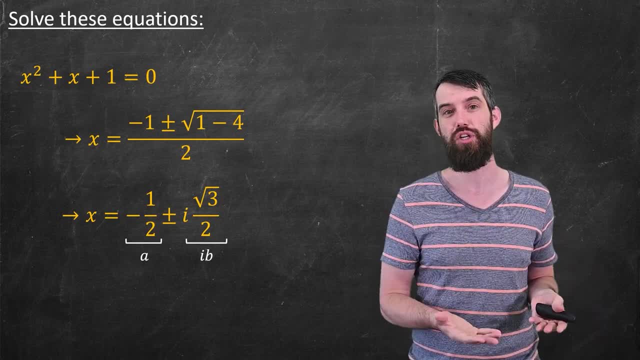 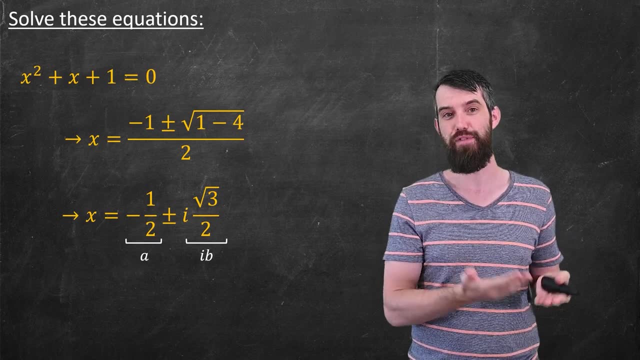 that does not have an i attached to it. I'm going to call that a in the future. And then there's something that's got an i times. well, root three over two in this case. I'm going to call that i in the future. And it's worth noting that the quadratic formula always works this way: It. 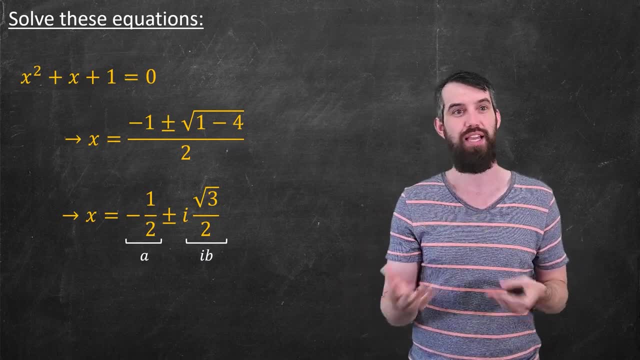 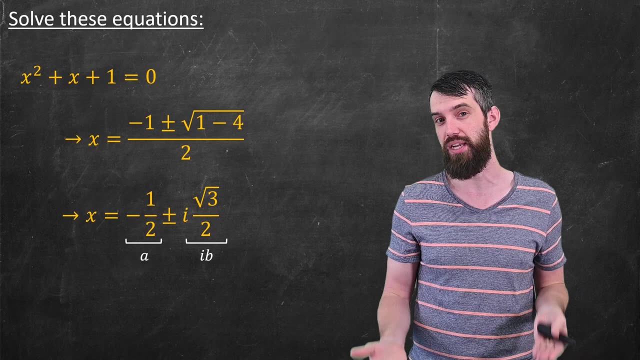 always has this square root. The square root's either positive, in which case it's just a real number, like we saw before, or the square root's negative, in which case we can factor out that negative and get an i in the way we've just done now. So this leads me to my definition. 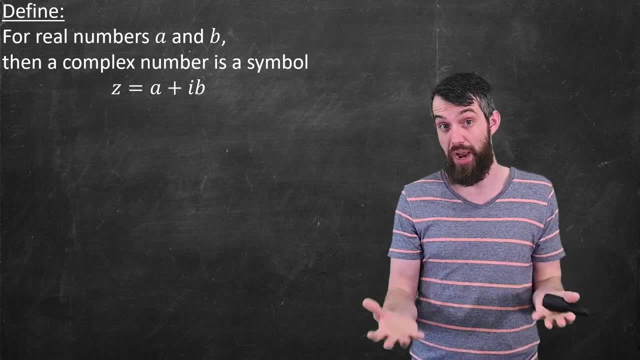 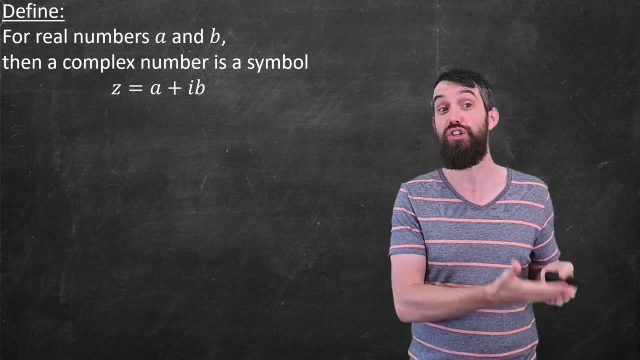 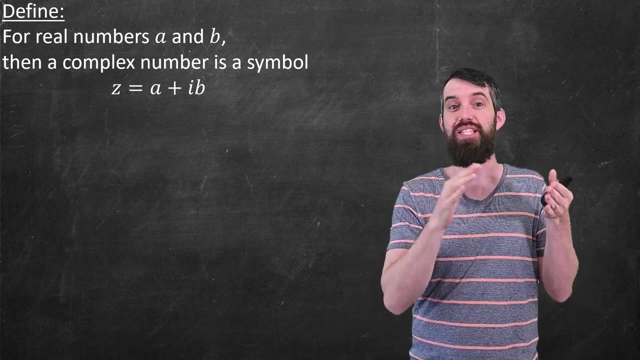 of complex numbers. The definition is that if you have two real numbers- and here a real number are things like integers or fractions, like three, sevenths, or irrational numbers like pi and e and root two- all of those collectively are real numbers- then a complex number is the. 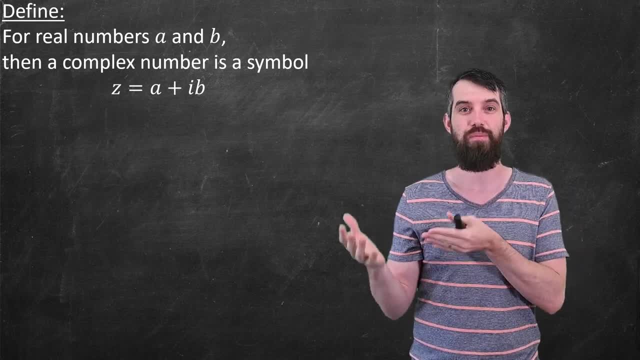 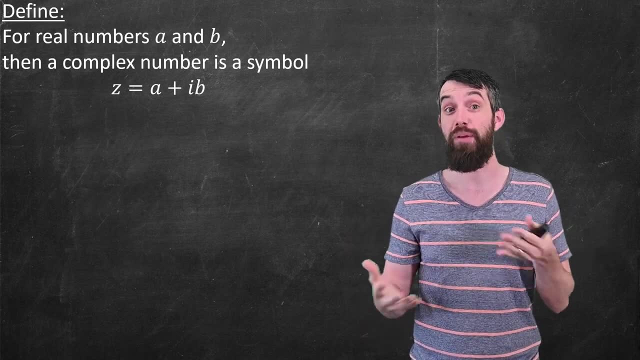 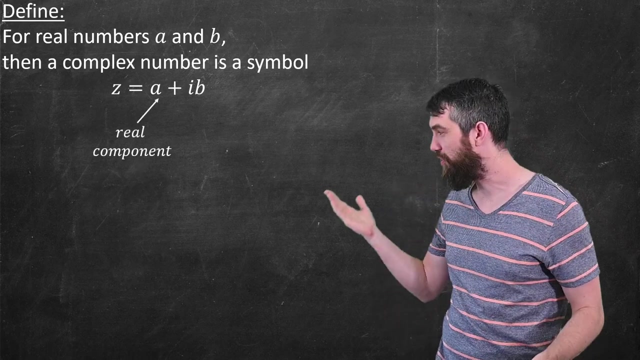 symbol z equals a plus i b. This is just defined to be the object. Things that look like that, like an a plus i b, often relabel them with shorthand as z, But either way those form complex numbers. I have some terminology around this. I call the a 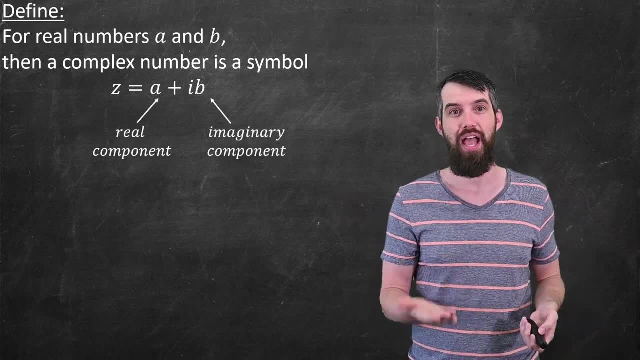 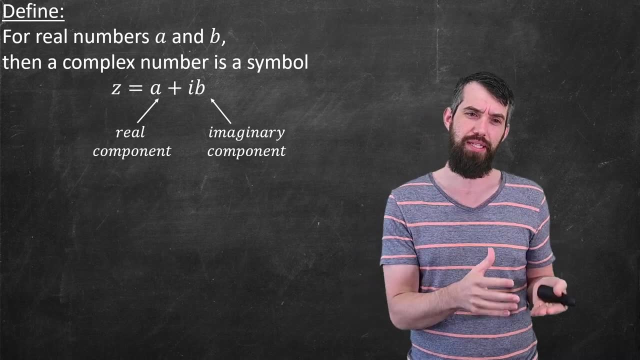 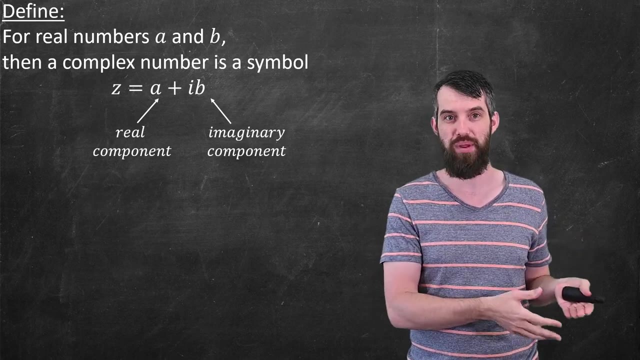 just the real component of it, because it's just a real number by itself. And I call b the imaginary component, That's the portion multiplied by the i. So the point is that I define complex numbers in this way because this is the type of format we got when we saw the quadratic formula. 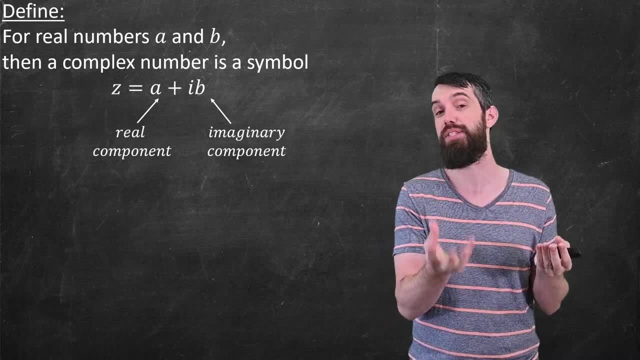 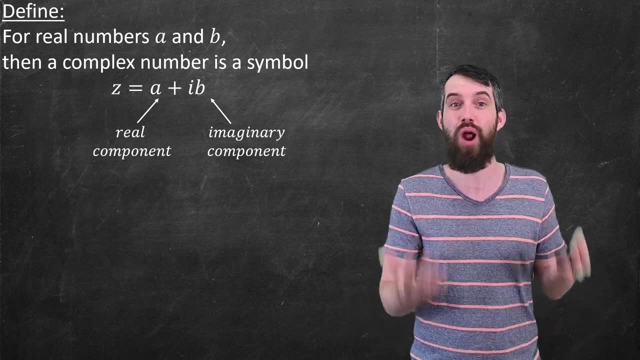 It looked like sort of a real number plus an i times some other real number. So we're going to sort of abstract it away and define the complex numbers this way. But now that I've defined them I have to define: what other properties do they have? So, for example, can you add two complex 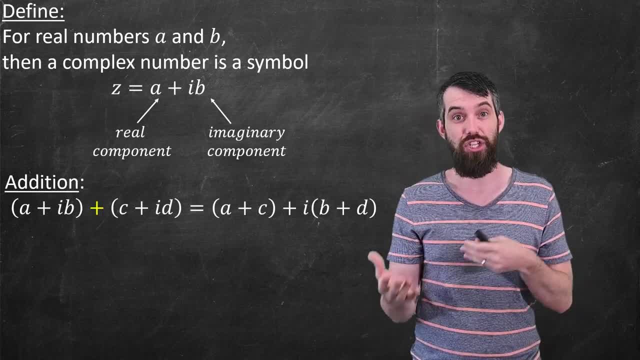 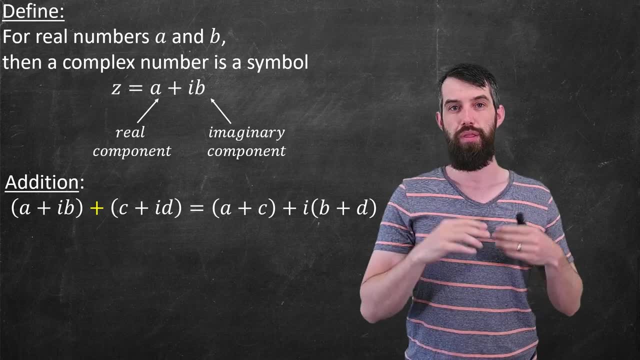 numbers. Well, we can do that. I'm going to say that the addition, the addition of two complex numbers, so an a plus an i b, and then I add to that a c plus an i d, The two real components, the a and the c, add together and give the new real component a plus. 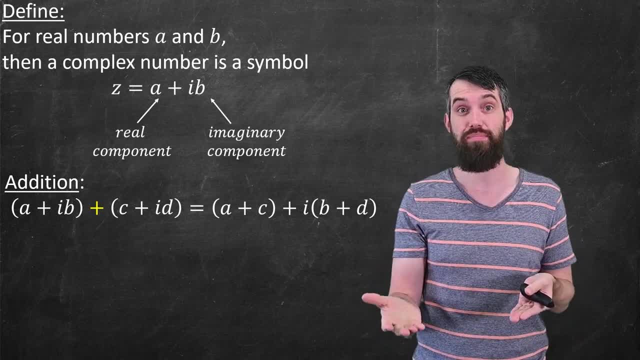 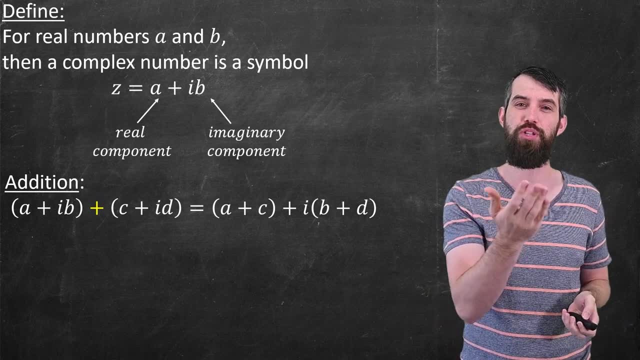 c And the two imaginary components, the b and the d, add together and give the new imaginary component b plus d. Seems a very natural definition of addition. to give, All right. What about multiplication? So I've got an a plus an i b and I now multiply it to a c plus an i d. Well, I'm going. 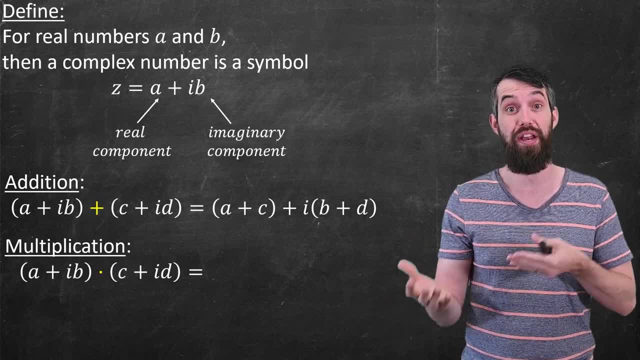 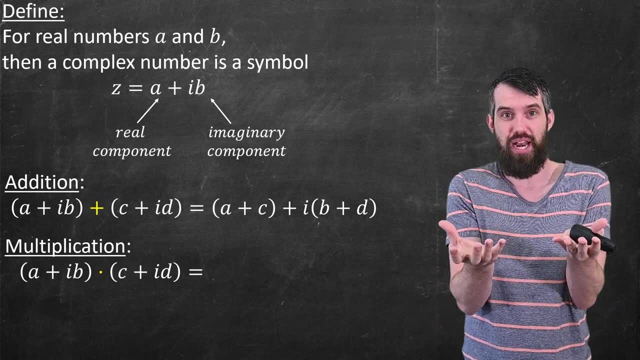 to imagine that my multiplication works sort of the same way it would if I had normal numbers. I'm going to have things like the distributivity law. So if I have these two different terms and I multiply them together, well, what am I going to get? We will define multiplication in such 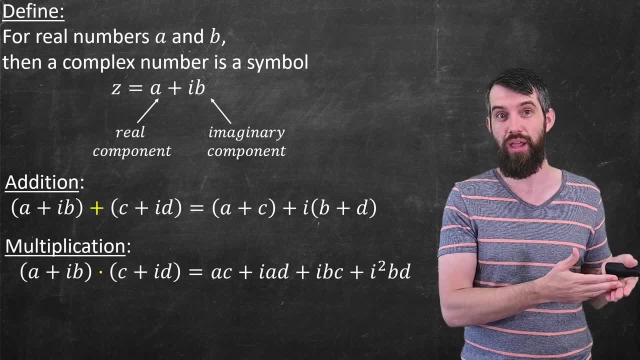 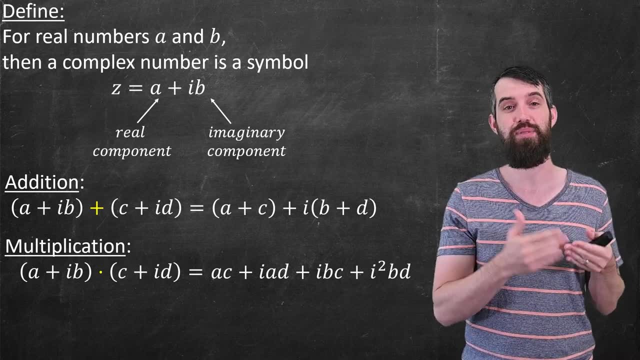 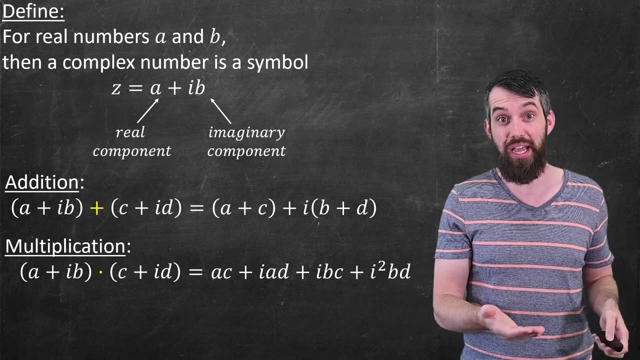 a way that it obeys the normal distributivity law. And then when you distribute these out, well, you get a c plus i, a d plus i, b, c plus i squared times- b d- Note here that i squared is 1. So I can just take that i squared and replace it with a negative And then recombining things. 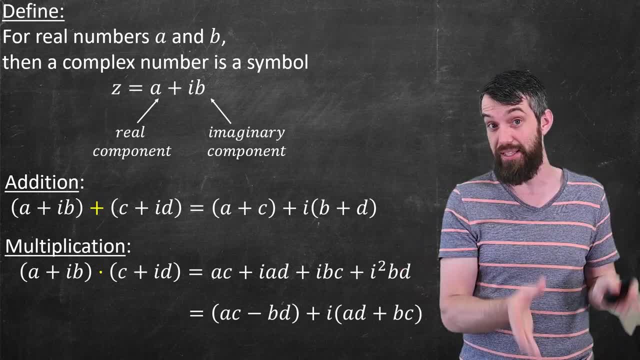 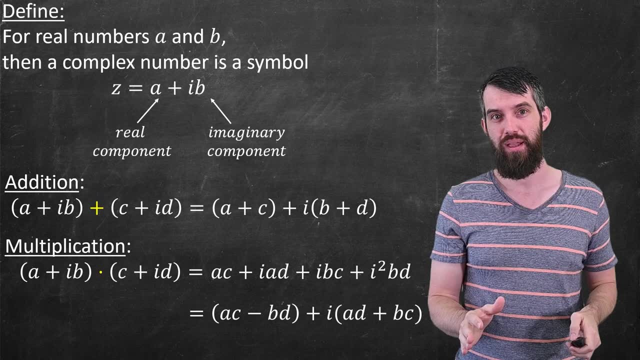 I get an a c minus b d. That's my real component, That's the stuff that doesn't have an i And the things that has an i is an a d plus b c. So that is my definition of multiplication. Now, I actually don't normally just memorize this, I just work it out each time. So if I 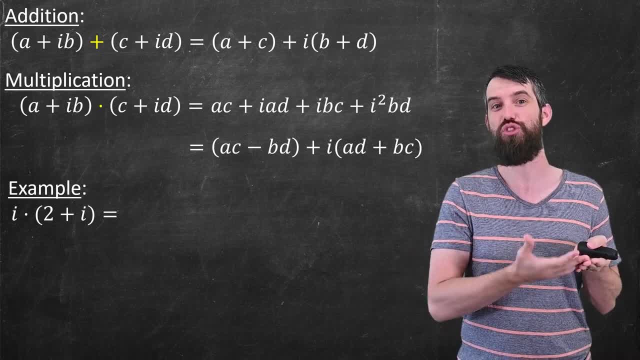 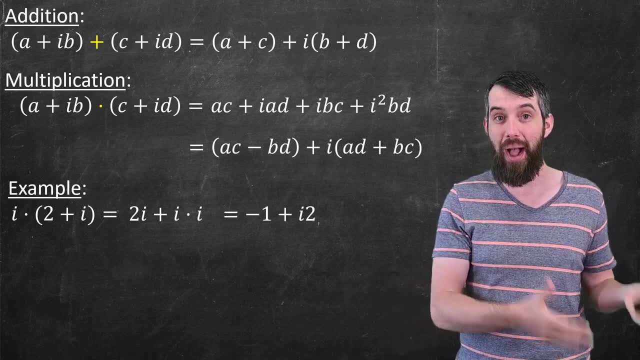 have an example. for example, i times 2 plus i, Well, I distribute the i across. This is going to give me 2 i plus i squared, And then i squared is minus 1.. And so I can't finally get the i squared. So I'm going to take the i squared And then I'm going to take the i squared. 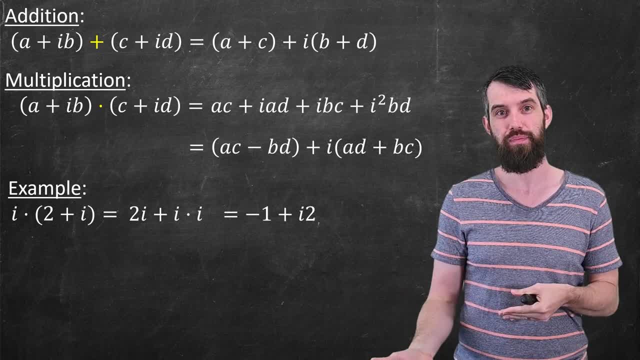 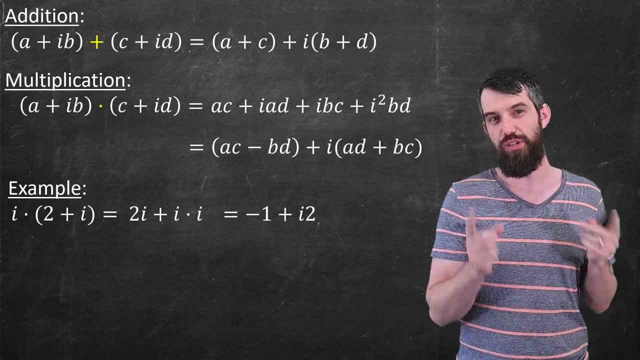 minus 1 plus 2 times i. This is the way I've written this in its standard form, as a complex number. Now, addition and multiplication are very familiar to us in other types of mathematical objects, like the real numbers, But there's one new operation that is a little bit different. that 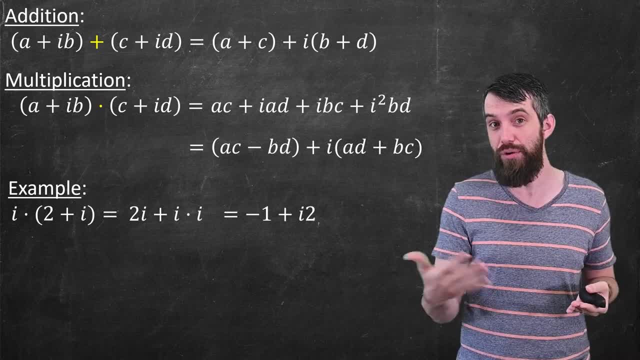 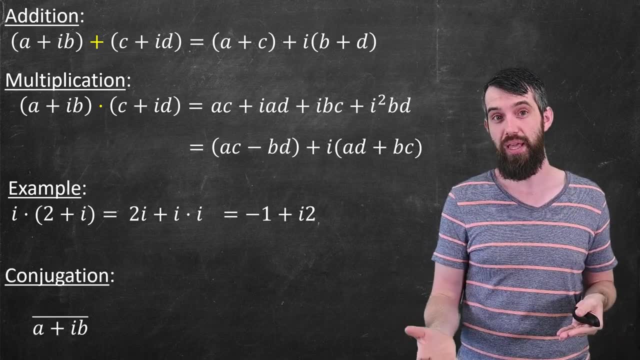 we don't have over, for example, just the integers, And this is called taking the complex conjugate. It's another definition of another new operation that one can do on complex numbers. Take the a plus i, b, And then you write a horizontal bar on top of it, And then the way. 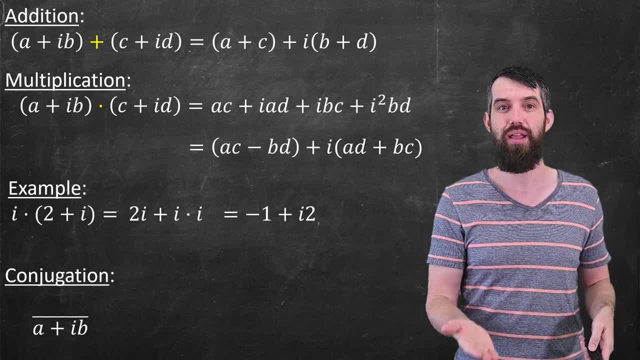 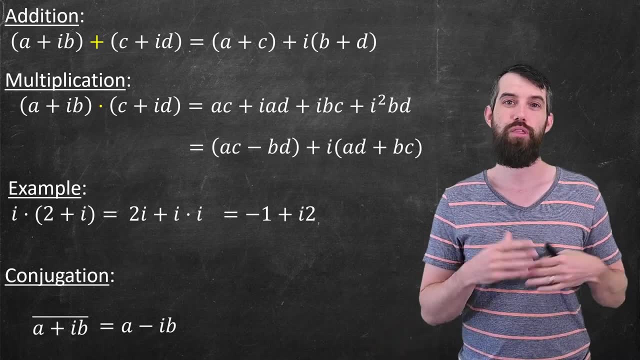 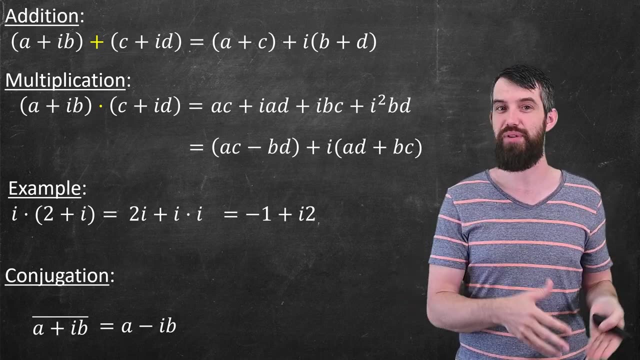 it's defined is that it just takes the imaginary component and makes it negative. So a plus i b conjugate is a minus i b. The reason why this is so useful is that in the quadratic formula you get a plus or minus a square root. So it's useful to have some notation to talk. 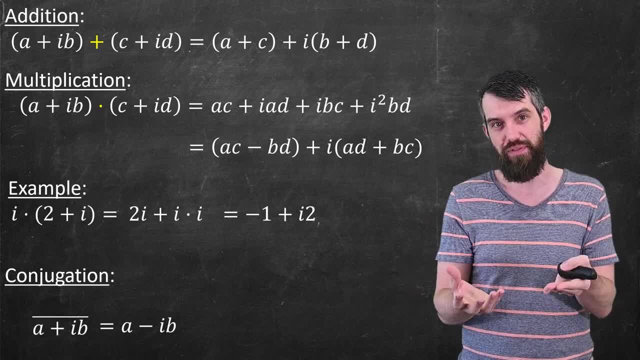 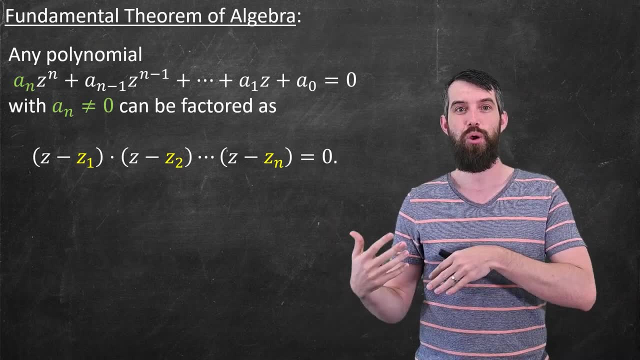 about when you've got the positive imaginary and the negative imaginary portion of this. So that's why we have this extra little bit of definition. Now, the way we define complex numbers was we were looking at the quadratic formula and we were sort of looking at the answers to the quadratic formula to motivate our definition of. 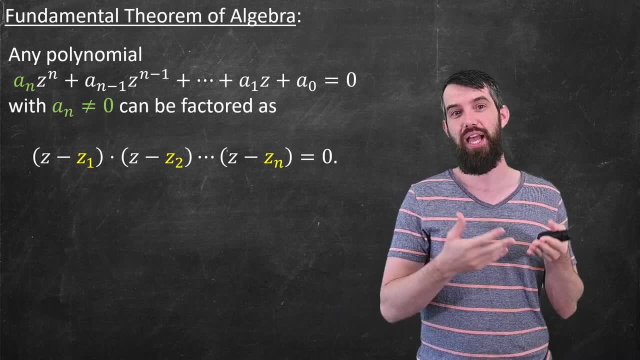 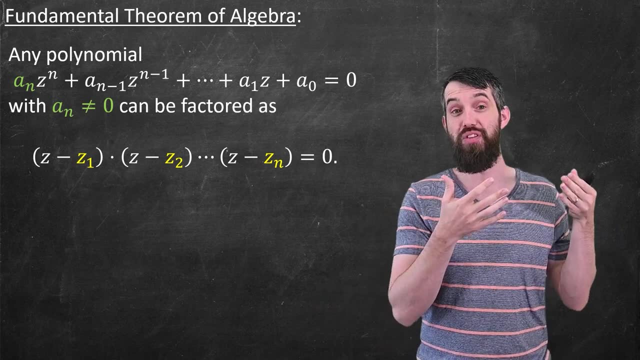 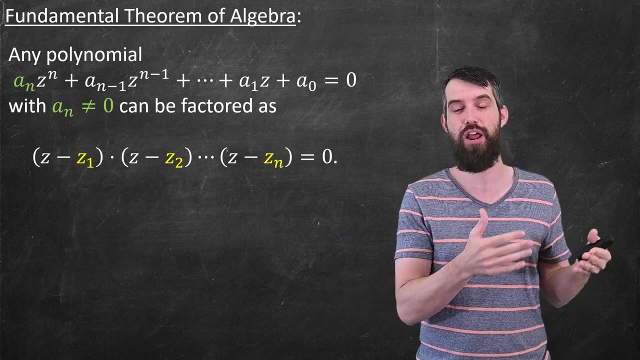 complex numbers, But what I want to observe here is that this actually works for any polynomial. Indeed, one of the most powerful theorems in mathematics is called the fundamental theorem of algebra, And basically what it says is that a degree n polynomial has exactly n roots. 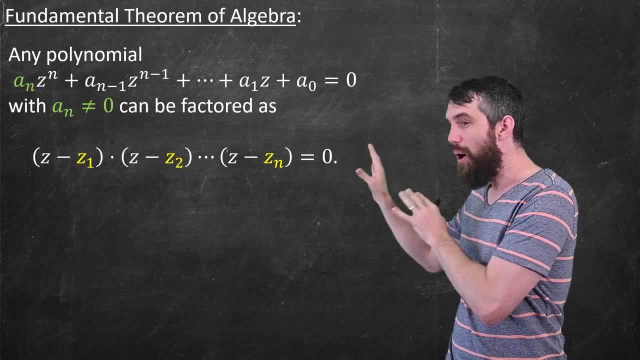 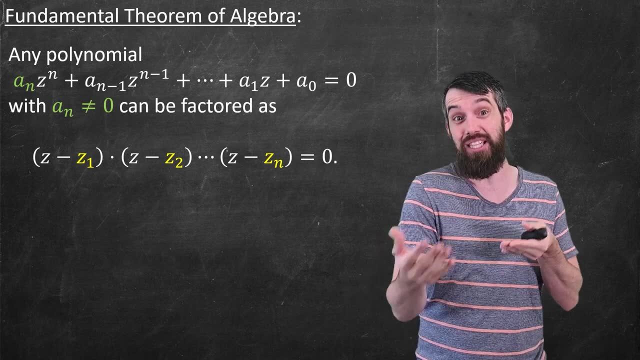 So, stepping through the language a little bit more more precisely, I start with a polynomial here where I write a sub n, that's just a coefficient, and then z to the n- Z instead of x here, because I'm going to imagine that my variables could be. 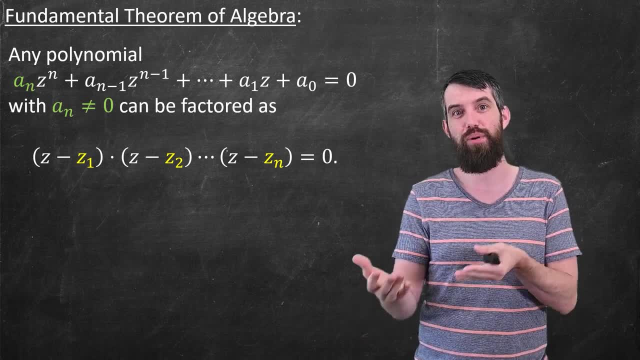 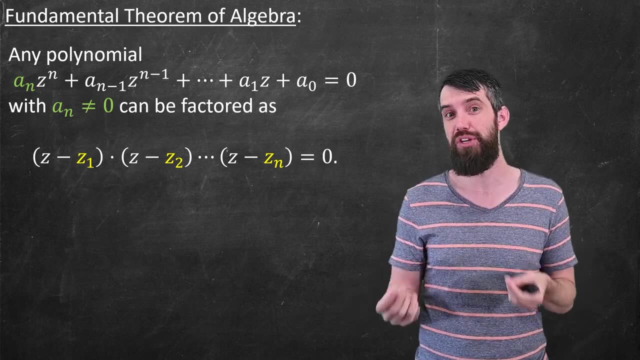 complex numbers and z is sort of the generic complex number where x is sort of the generic real number. But nevertheless, if you have some polynomial, that is a degree n. what I mean by degree n is that it's highest power is n, or a way to say that, is that a, n, the coefficient of 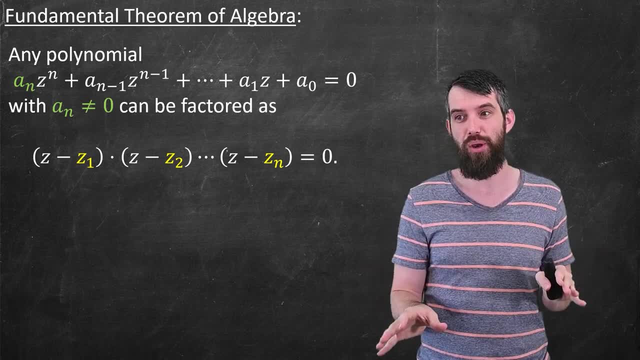 the highest power term is non-negotiable, and that's just the cost of the cart. And if I write a 0. Nevertheless, you have this degree n polynomial, and then you can factor that as well: z minus z1,. 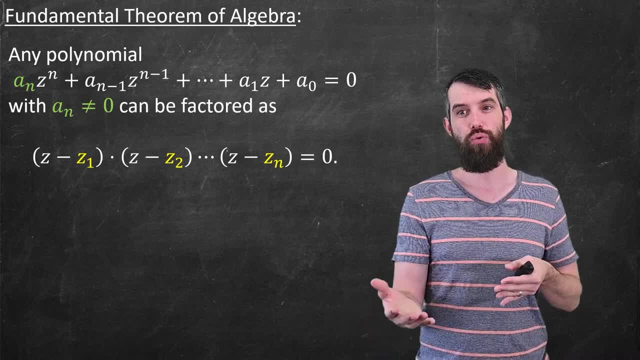 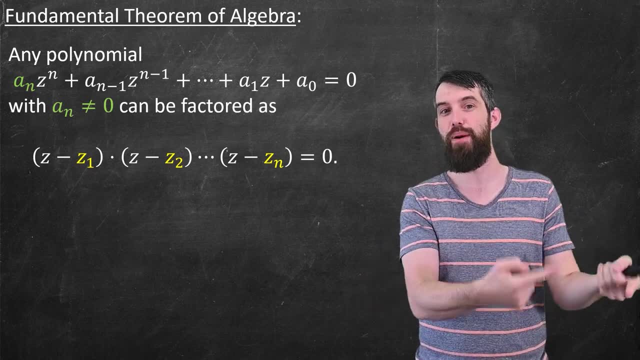 z minus z2, z minus z3, and so forth. So your roots, your solutions, the complex numbers that you can plug into that polynomial and get 0 are the z1, the z2, the z3.. What the theorem is really. 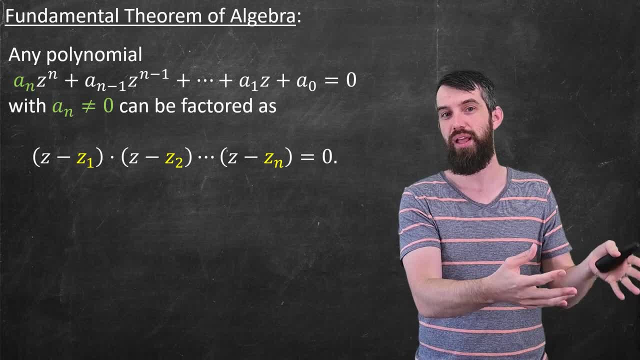 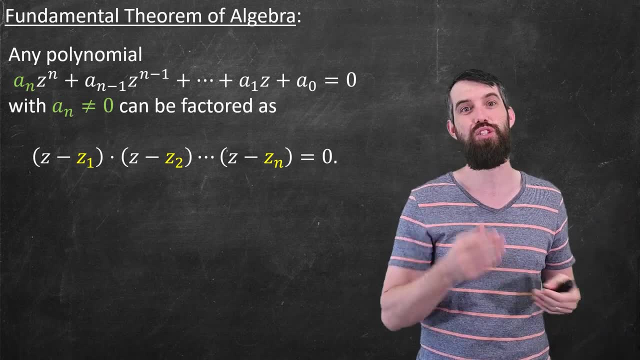 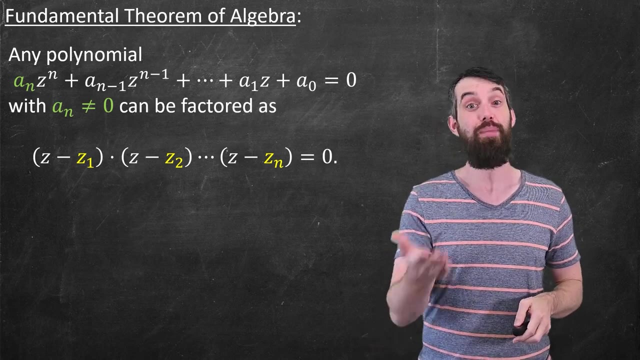 saying is there is n of them. So if you have an n degree polynomial, then you get n complex solutions. This is not the case with real numbers, even that x squared equal to minus 1. That's a degree 2 polynomial, but it has no real solutions. Okay, let's see one example. Let me take for 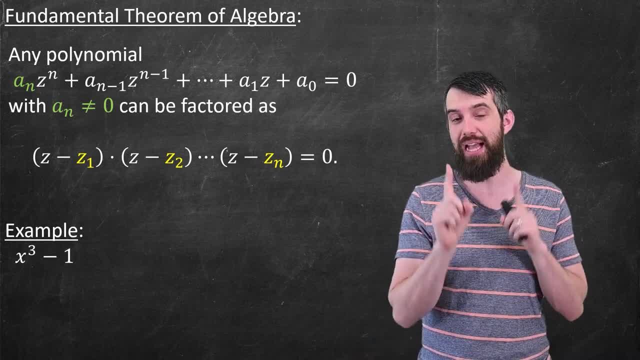 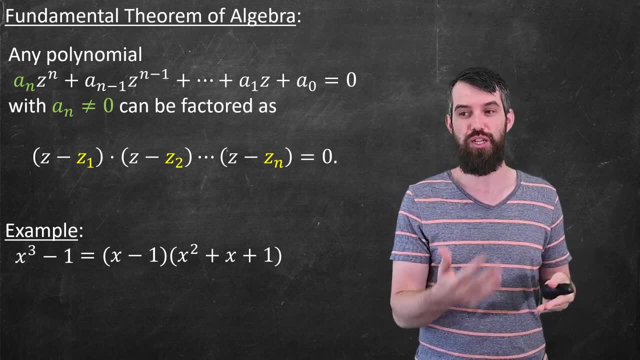 instance x cubed minus 1.. So not x squared now, it's x cubed minus 1.. And I can factor this. you can verify by multiplying it out, if you wish- that this is equal to x minus 1 times x squared plus x.